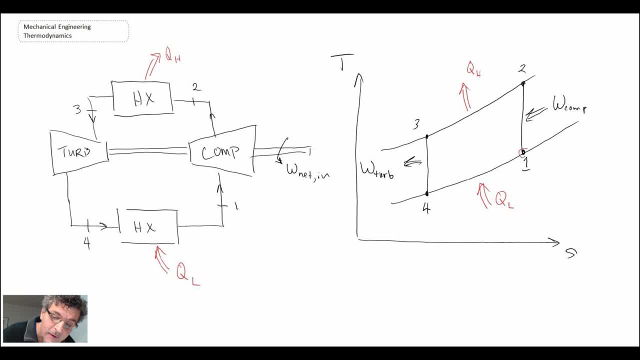 we start off with air. it could be at atmospheric temperature and pressure, it could be a slightly different condition, but we go through a compression process and after the compression process the air heats up. we do work on it. it then goes into a heat exchanger at state two and then that comes down to state three, after we reject thermal energy or 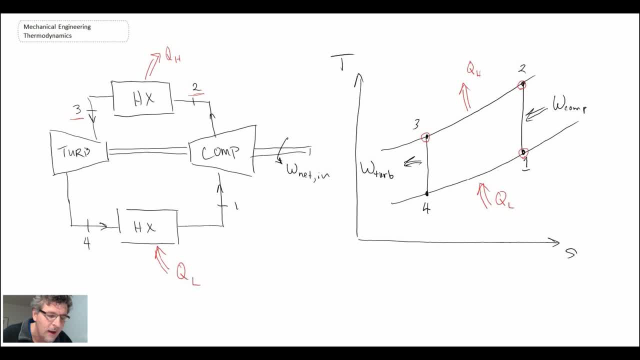 heat to the surrounding environment, and so that's what's going on there. we then go into a turbine, we recover some of the compression work and by expanding or cooling we come out at state four. we then go into another heat exchanger whereby we absorb thermal energy from whatever environment. 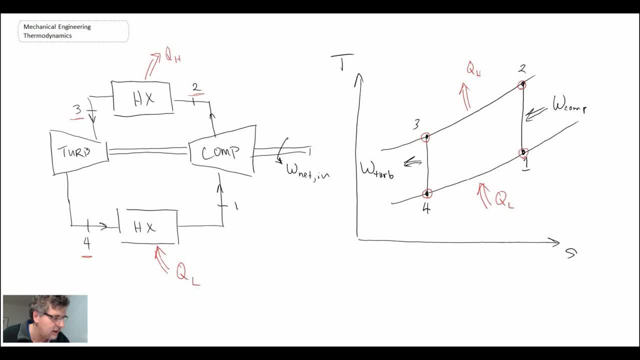 it is that we are trying to cool, and so that gives us an idea as to what the cycle looks like. let's take a look at the coefficient of performance. so our desired output is the heat transfer from whatever a low temperature source we have and the amount of work that we're putting in. we put in work into the compressor. 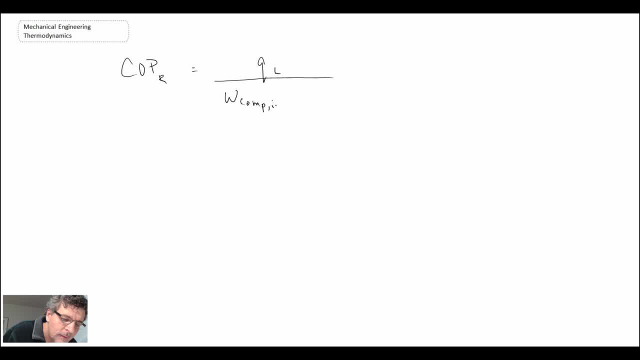 and we recover some work out of the turbine, and so it's the difference between those two would be the work in, and then enthalpy differences are where we get all the different parameters from. so for QL it would be the enthalpy change between one and four. 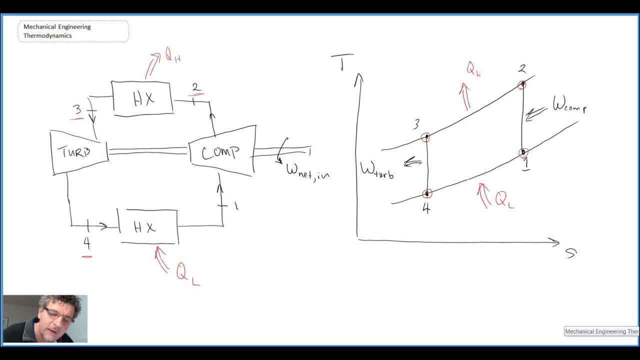 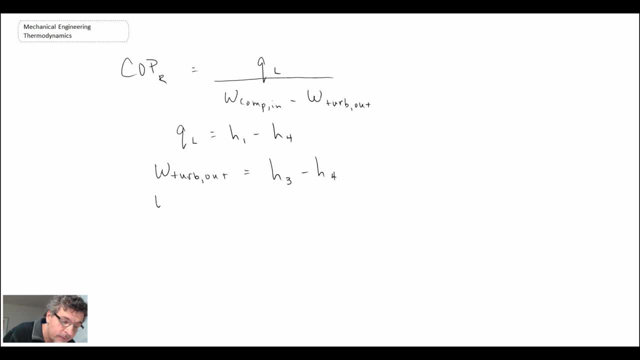 Curbine out would be the change in enthalpy between states three and four, and then one and two for the compressor in. Now, one common application where this gas refrigeration cycle is quite often used is inside of aircraft, and it's used for air conditioning within aircraft, either heating or cooling the air. 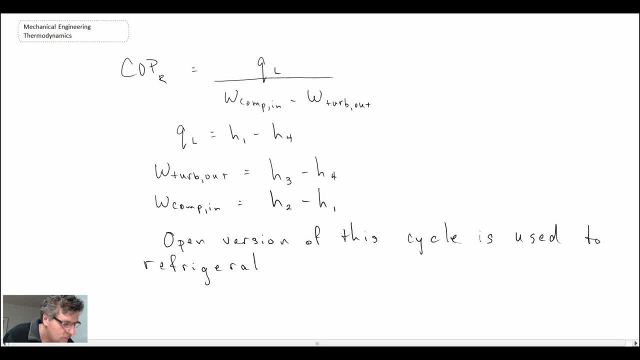 And the advantage is is that it has a very light weight. Some older aircraft used to use refrigerants, but in recent years- I think the 707 was one of those, but in recent years all the aircraft were refrigerated. Some older aircraft have used this cycle in order to condition the air.